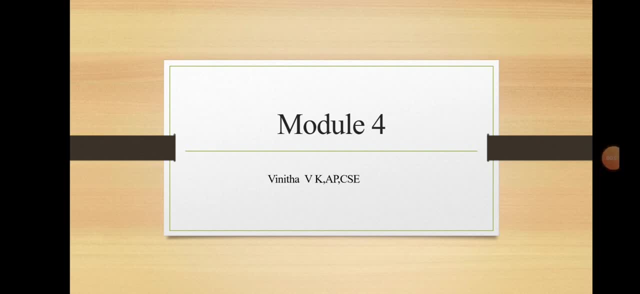 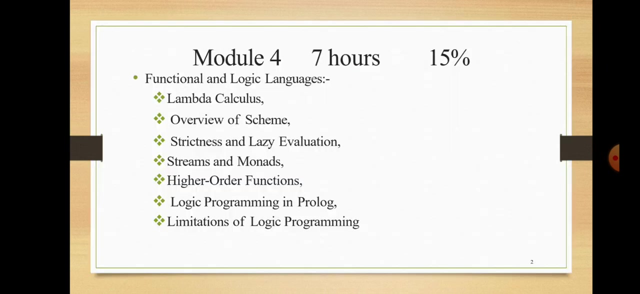 hi, students, in this video we are going to start the fourth module of programming paradigms. okay, the fourth module mainly deals with functional programming language and logic programming language. okay, so these are the main contents of fourth module. the main content are functional and logic languages. within that we have to study whatever the lambda calculus overview. 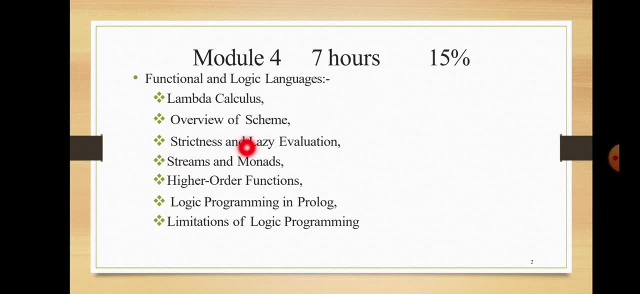 of the language scheme, then strictness at lazy evaluation stream and monads, higher order functions. logic programming language in prologue, then limitations of logic programming. okay, so the main heading behind this module is functional and logic programming language and logic programming language in prologue and logic programming language. so we have to start with the basic concepts of 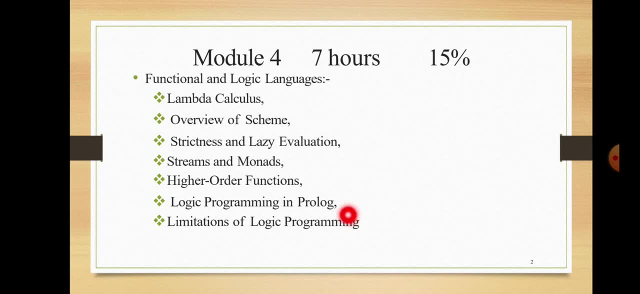 functional language. okay, so far we have already discussed, we have already learned some procedure languages, some objitorial languages, all that things we have learned, but we have never met or come across the functional language. okay, so in this module we are going to discuss about some overview or some or some basic concepts of functional programming language and logicんですaly. okay, lag ih. yes, and we, we will start with the Bunuk, except of which we have accepted, and so that we all understand very good the general logic of functions, the language. okay, so in this module we are going to discuss about some overview or some basic concepts of poolслr, is ok. so in this module we are going 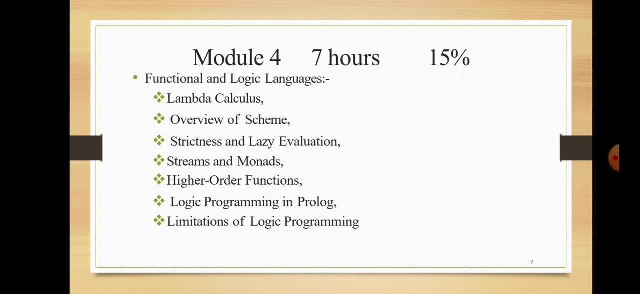 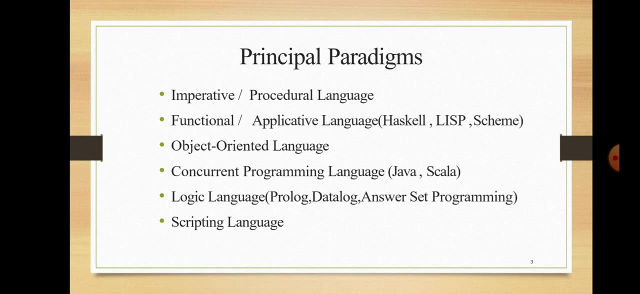 functional programming language. okay, so these are the basic type of languages which we are using for programming. okay, imperative or procedural language, then functional or applicative language, then object-oriented languages, then concurrent programming languages, logic languages and scripting languages. okay, so these are the types of, or the programming languages can be classified. 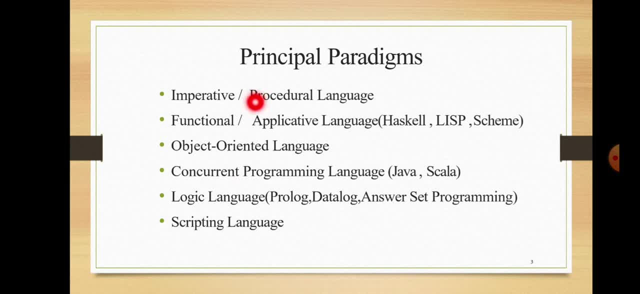 into any of these types. okay, so we have already studied procedural languages. for example, C is a procedural language. okay, so there we are writing everything as procedures or statements. statements are written in C, so it is an example of procedural language. okay. next is next category is functional. 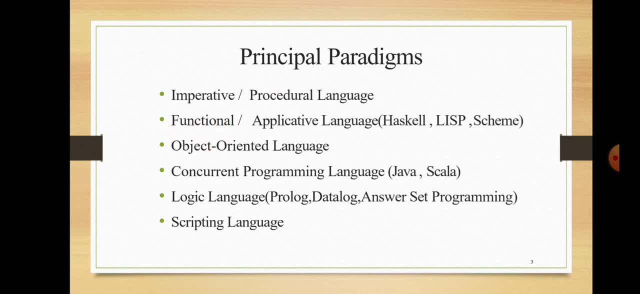 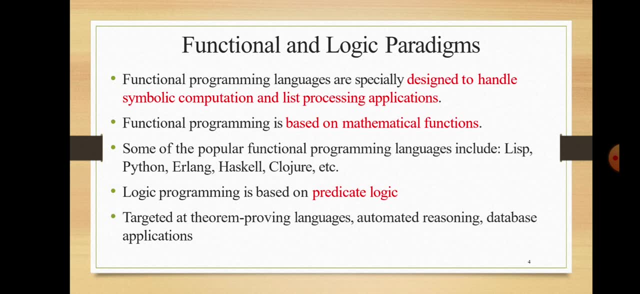 language, which we are going to discuss in this module. okay, so what are the specialty of functional language? functional programming language are especially designed to handle symbolic computations and list processing applications. okay, so functional programming languages are specially designed to handle symbolic computations means what we use? symbols, and that is, for example, lambda, like symbols. okay, 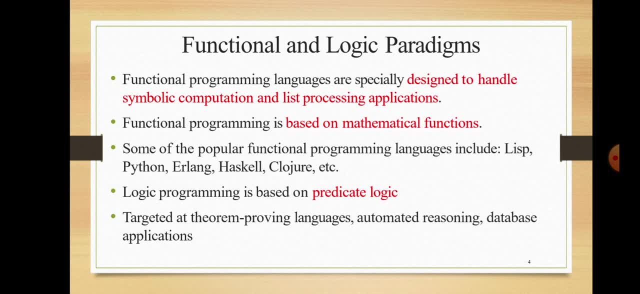 symbols and also for list processes. list is a particular data type which takes a collection of statement values as input and sometimes produce a collection of value as the output. okay, so for all these purpose we use functional programming language. okay, the basic idea behind functional programming is mathematical functions itself: maxing out of the number you say, Jena. 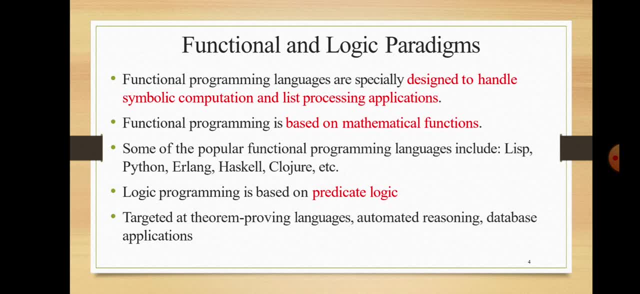 mathematics lay uses in a same functions as an honor, a, the basic concept in order in the functional programming language, in the concept in the writing of the other one data. it is used to design symbolic computations in the parinada okay, number of max nagata there in the equations of the name, equations, and I'm just addition. 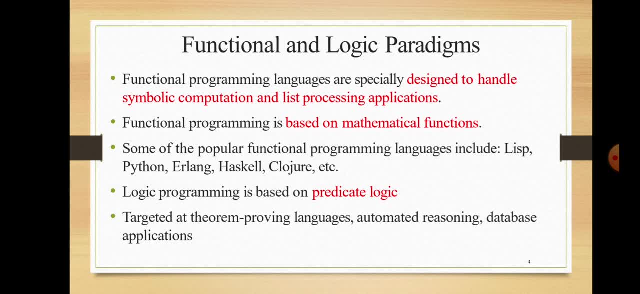 subtraction, multiplication, divisions are the martyred. other symbols, name computer am. in order to do such computations, we have to use functional programming language. okay, so some of the popular functional programming language may include LISP, Python, Haskell, scheme. all these are examples of functional programming languages. okay, in this podium we have to discuss one such functional programming. 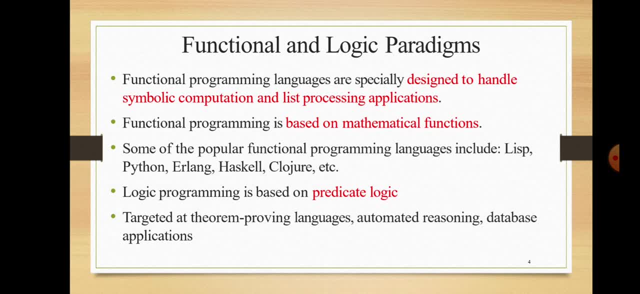 language, that is, scheme. next, logic programming language is based on the predicate logic. so far you have, I think in the third semester you had studied in discrete mathematics about the logics, predicates and so on. okay, so in order to perform such computations we have to use the logic programming languages. it 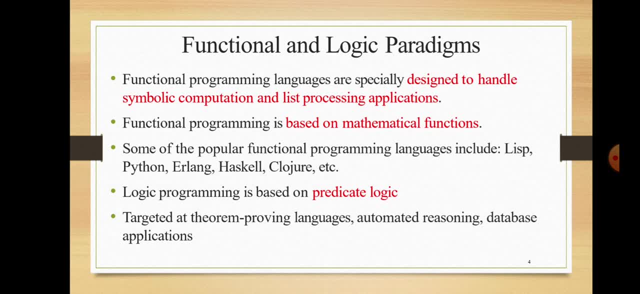 mainly focused on theorem, proving automatic reasoning, database applications, etc. okay, so we mainly use logic programming language for proving the theorems, then for automated reasoning, then database applications, and for all these purpose we use logic programming language. okay, so the main purpose of functional programming languages it. 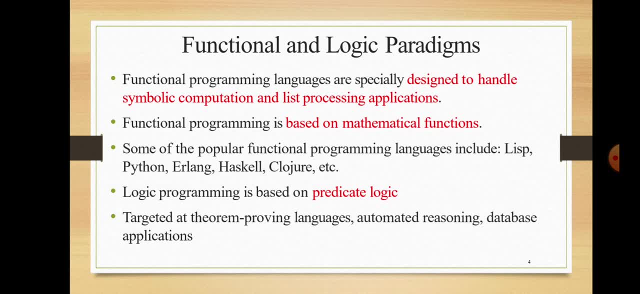 used to deal with symbolic computations and also for list processing applications. okay, the basic idea behind functional programming languages mathematical functions itself. okay, some of the language which support functional programming are Lisp, then Haskell, Python. why Python is a functional programming language? it is simpler to programming. list processing is very easy in Python. 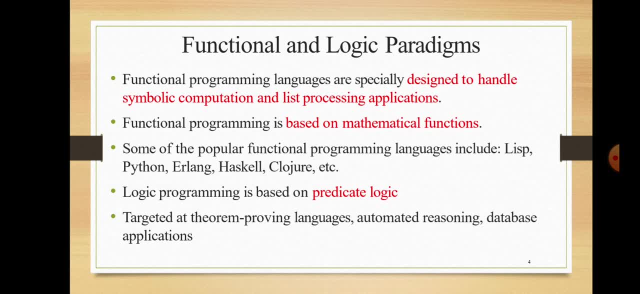 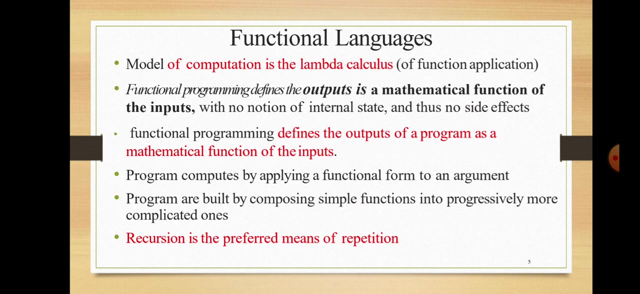 okay. so then we studied: what is logic programming. the basic idea behind logic programming, or the main concept, is predicate logic itself okay, and it is mainly used for proving the theorems, then for automatic reasoning, the database applications, etc. now we are going to study or look into deep about. 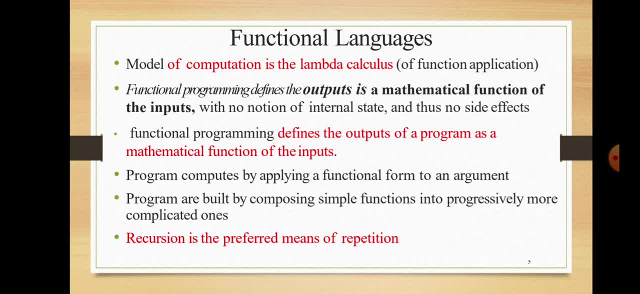 a functional language. okay, so the model of usted computation is the lambda calculus, The computation model used by functional languages, lambda calculus In the model. we will discuss in deep what this lambda calculus. Okay, So the mode of computation used in functional programming is termed as lambda calculus, Functional programming. 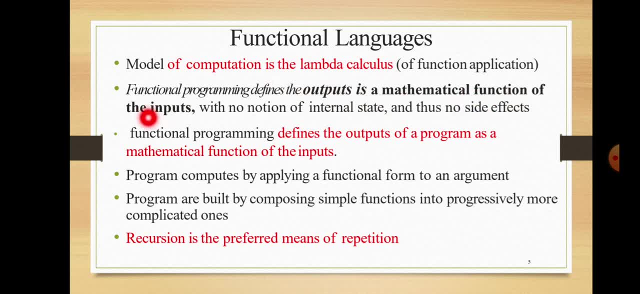 defines the output is a mathematical function of the input, with no notion of internal states and thus no side effects. So in the case of functional programming language, output is always a function of the input. So there is no internal states In between input and output. there is no internal states. since there is no such internal states, there is. 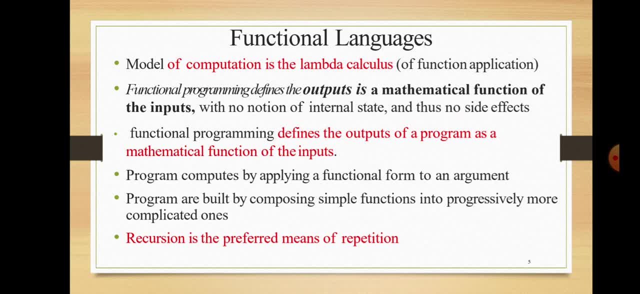 no side effect. Okay, So here, always, the output will be a function of the input. Okay, So functional programming defines the output of a program as a mathematical function of the input. Program computes by applying a function form to an argument. we apply a function to these arguments. 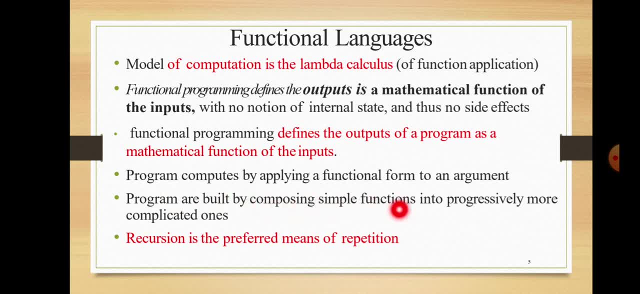 Programs are built by composing simple functions into progressive more complicated ones. So how do we create functional programs? By creating simple programs. we will bind them together to form a complicated one. We will not solve a big problem in the same way. 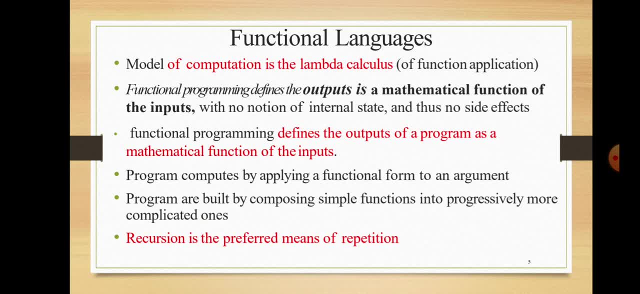 We will divide it into modules and we will implement them as smaller ones. We will use simple functions to implement each one of them. Lastly, we will tie them together to form a solution to the original problem. Input is No, sorry. Output is. 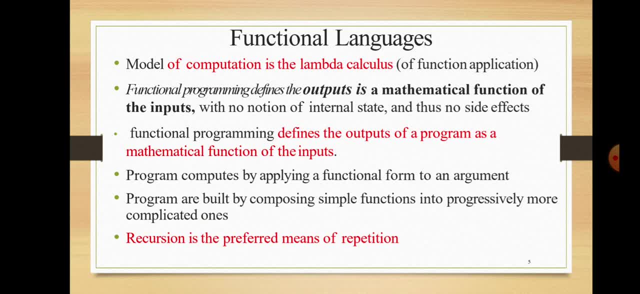 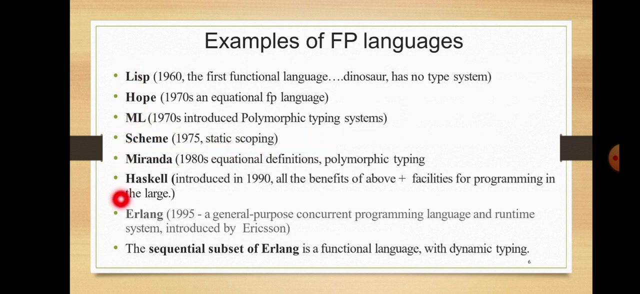 It will be the function of an input. Recursion is the preferred mean of repetition In functional programming. we will use the same recursive mode. So far, these are the various types of functional programming language. The first functional programming language is Lisp. 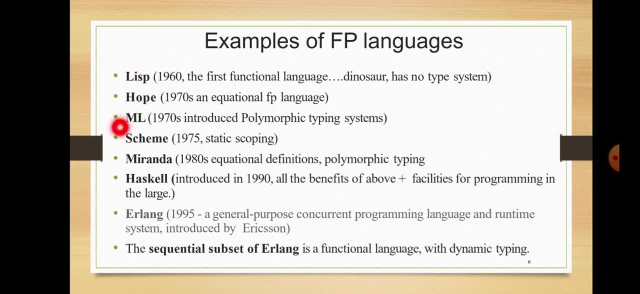 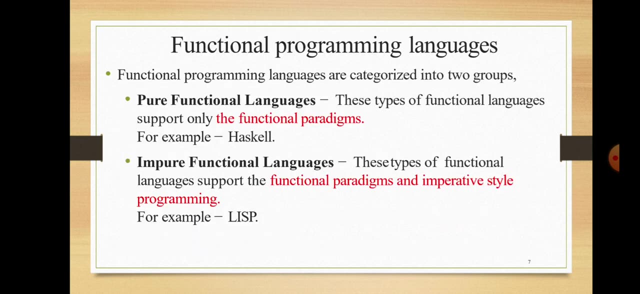 Then comes the HOPE, then ML, then Scheme, Miranda, Haskell, Erlang. The sequence subset of Erlang is also a functional programming language, So the first functional programming language is Lisp. The functional programming languages are mainly categorized into two groups. 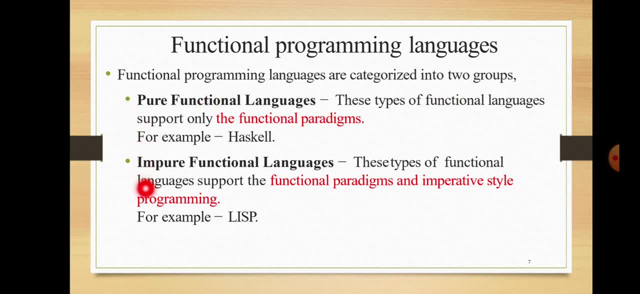 Pure functional programming language and impure functional programming language. Pure functional programming language means what It means. these types of functional languages support only the functional paradigms. The programming, The functional language is said to be pure if it supports only the functional paradigms. 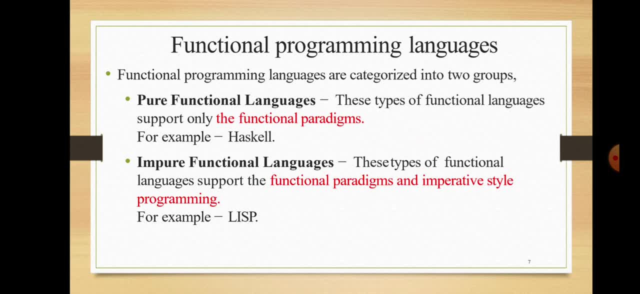 For example Haskell. Haskell is a pure functional language. These are the languages that only support the paradigms of functional programming languages. The functional languages that only support the functional paradigms are called Pure functional languages, For example Haskell. Impure functional language means what? 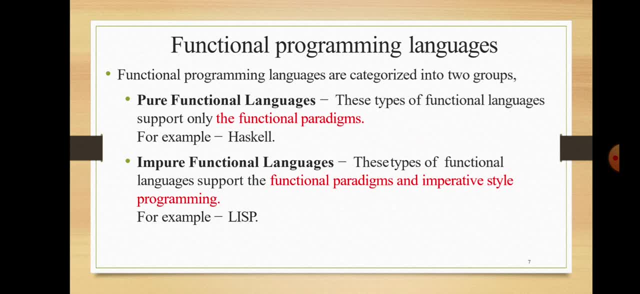 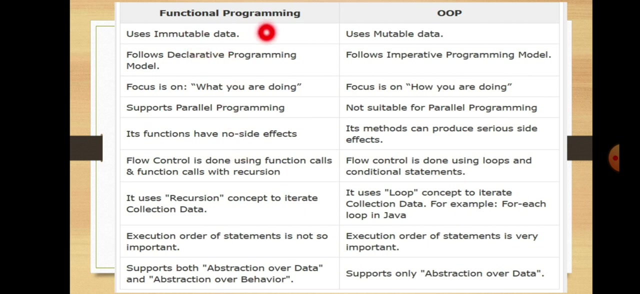 It supports both functional paradigms and also imperative style programming, That is, we can write it as a procedure, but we can also use the functional paradigms. The functional languages that support such combinations are called Imperative functional languages, which is, for example, LISP. okay, this is the main difference between functional 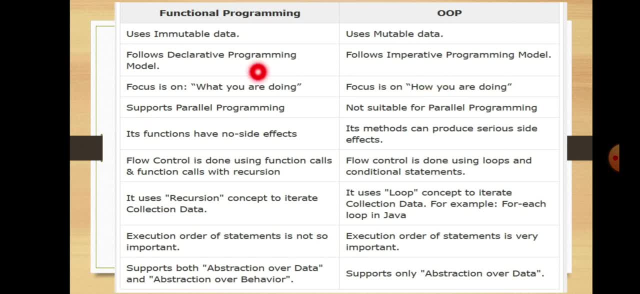 programming and OOPs. I am just going to read it out here. It uses immutable data. here it uses mutable data. then functional means: it follows declarative programming model. OOPs: it follows imperative programming model and then it focuses on what are you doing? Functional language: always focus on what you are. 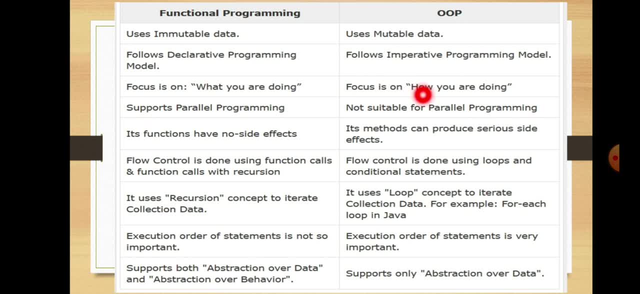 doing OOPs mainly depends on how you are doing. then support parallel programming. ooops, it is not suitable for parallel programming. then in the case of functional programming, the function has no side effects. Why? Because it does not have здistaments. Its mother can produce serious 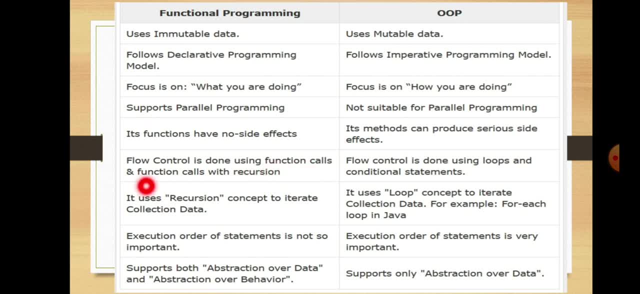 side effects. Flow control is known, done using function calls and function calls with recursions. Here flow control is used is done using loops and conditional statements. It uses recursion concept to iterate collection data. It uses loop concept to iterate collection data. For example, for each loop in java. 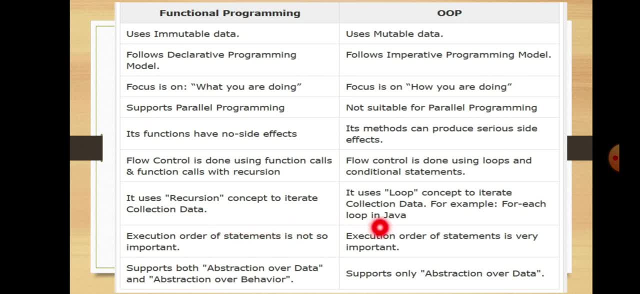 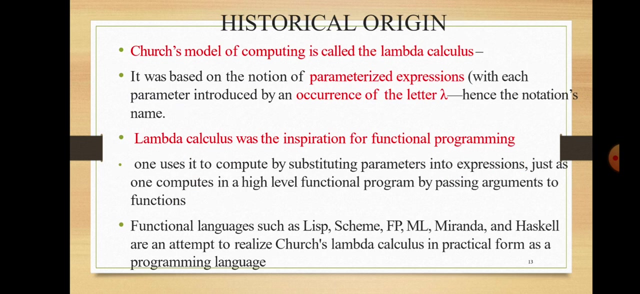 Then execution order of statement is not so important, but here execution order of statement is very important. Next is: support both abstraction over data and abstraction over behavior. Here it support only abstraction on data. You just go through these points, Okay. Now we are going to discuss some historic history behind the functional language. Okay, 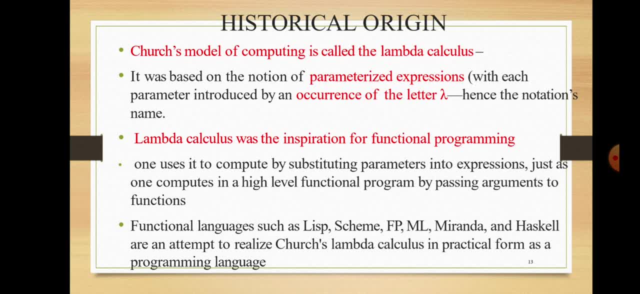 We have already discussed functional programming language. It will take collection of values as input and produce another collection of values, output. Okay, Behind this are some mathematical functions. Suppose we are taking an input, Let us not say a mathematical function as in the modern dictionary, but it is the mathematical function of by an input. Well, the mathematical function behind the function of a function. they will generalize this in two words: The function for input are some mathematical functions. How basic is the mathematical function of the function of input? After which it will pop the value which is equals to 1 backwards here, And the. 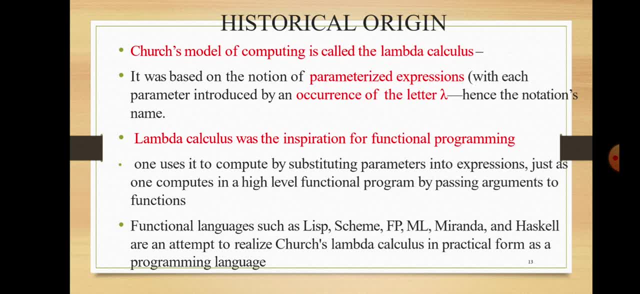 Falbertian method is taken in that and after that as an alternating. So now the function needs to. journalists functions apply to the initiation. I'm a candidate. no output number. produce a. no apa. are you do functional programming in day, basically where the computation in 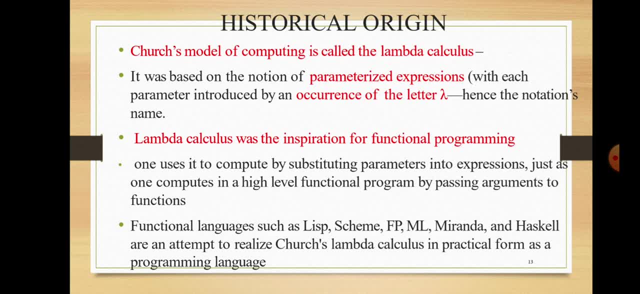 a blend, the term Jadoo, lambda calculus in the term Jadoo. okay, so this lambda calculus, in the parana, our model, is introduced by shorts. okay, so model of computing is called the lambda calculus. it was based on the notation of parametrized expressions. okay, then, in the trist expressions: 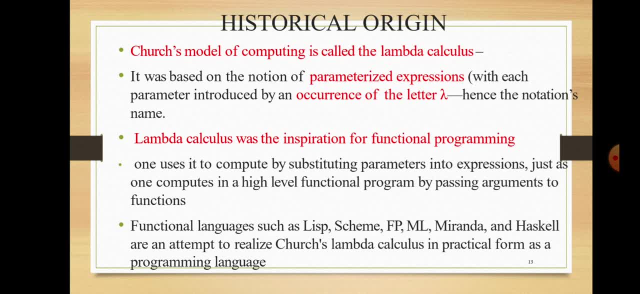 there's a parameters within the expressions. parameters or to cool even the expressions near and then the marina, the lambda calculus, a you do parameters. no, to cool even expressions in the expressions are on a number, lambda calculus, the basic notion, or another, okay, lambda calculus was the inspiration. 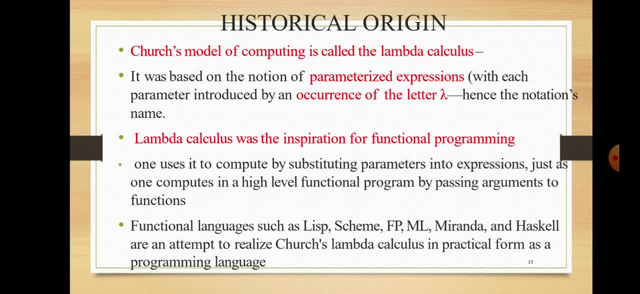 for programming language in general, a lambda calculus concept of another go, to put in the main in go to one of the functional programming language. because lambda calculus is the mode of operation behind functional programming language. one uses to compute by substituting parameters in the expression, just as one compute in a high-level functional. 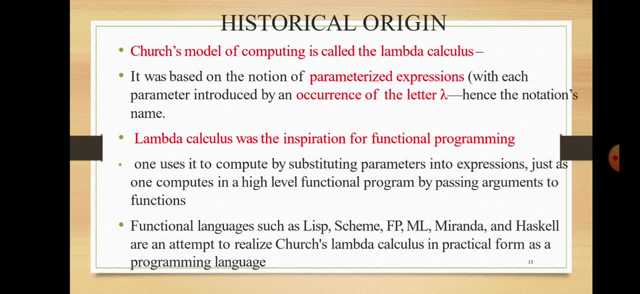 program by passing arguments to the functions. numbers are there now. if a secret, I'm running the same. if we're a function function call or no, I'm gonna say the function call, not the number of parameters, in that parameters is termed as formal parameters. I've, I'm actually in the 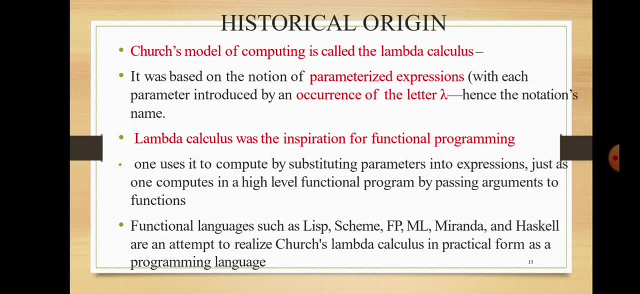 general formula parameters, then I'm gonna function, declare either can ever down. oh, I think I'll define. say they can never are. no, I would have gone to when they are. function for my parameters. now I'm going to pass it. I reckon I'm gonna output to produce in the same guy. I'm telling you what I'm using the number. 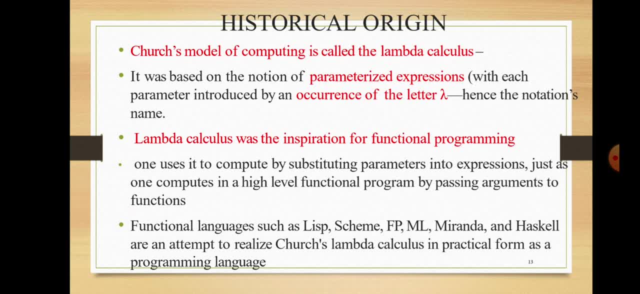 of our new lambda calculus, not in the bar and other. it is a parametrized expressions. so parameter plus expression around lambda calculus parameter number would. they should know the argument, argument in the foreign, the formal parameter, a formal parameter, an expression on, and then expression means the statement that has to be executed behind. this function is our function. 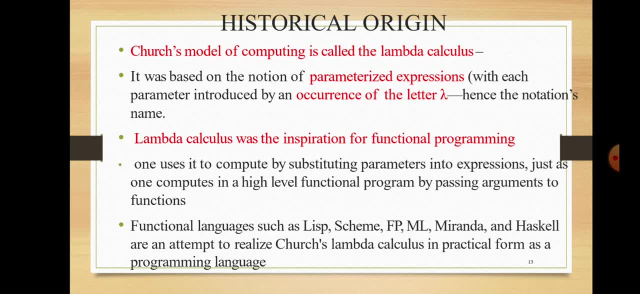 content animal say. you know the expression, the one with this either. okay, I put just to number I parameter. may I expression load to pass a move which is similar to a function called in the procedural language? okay, functional languages such as LISP, scheme, FL, ML, Miranda and Haskell are an attempt to. 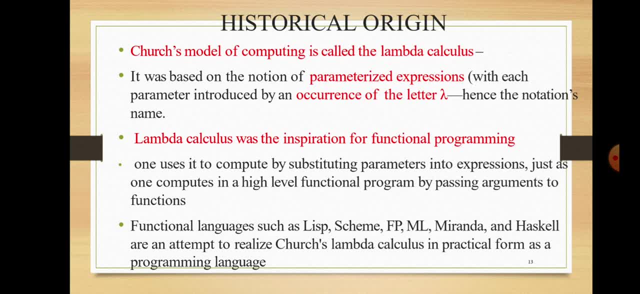 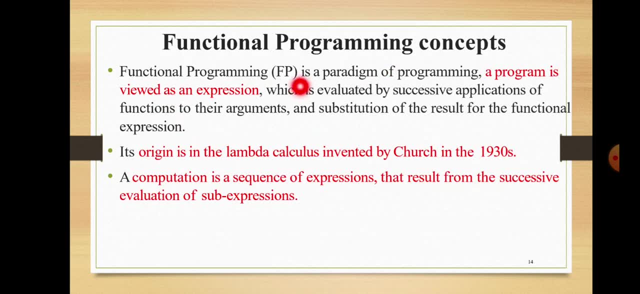 realize just lambda calculus in practice form as a programming language. okay, functional programming is a paradigms of programming. a program is used as an expression which is evaluated by successive application of functions to the arguments and substitution of the result for the function expressions. its O G is in the lambda calculus invented by church. which are you actually you? 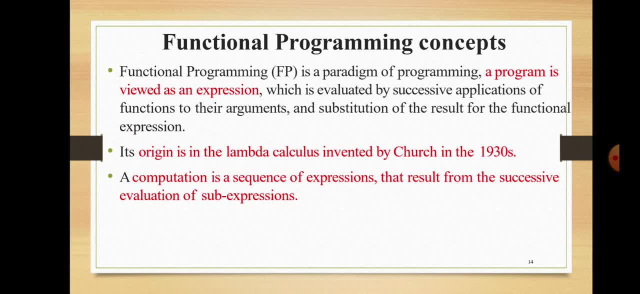 functional programming. and when the concept of Iran, like I didn't in Donna, you do lambda calculus in the bar, in the notion, the oru importance of the container. now to our model. what of computations uses a don't are either a concept, one of the name functional programming language, one of the name, a. 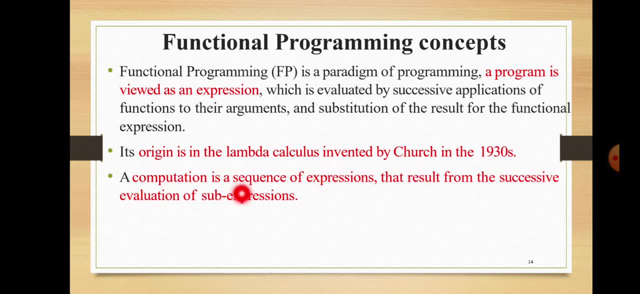 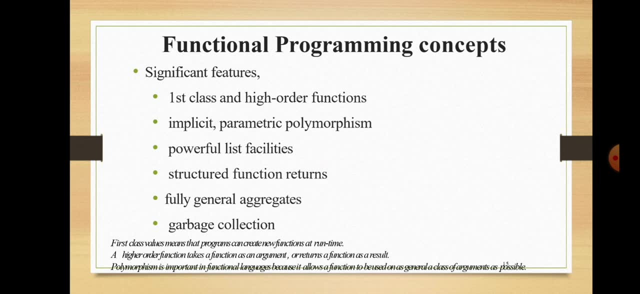 computation is a sequence of expressions that result from the success evaluation of sub-expressions. now we are going to the silent features of significant features of functional programming languages, and the first feature is first class and higher order function. first class function and higher order function: what does it mean? first class function means what in the channel. it mean we can, we can. 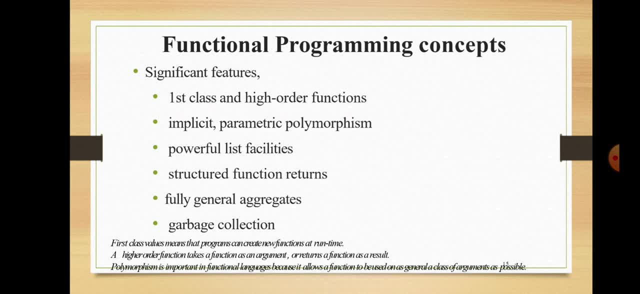 We are learning this word deeply. If we say the definition of this word, that program can create new functions at runtime. That means we are running a program, We are producing a lot of inputs. Output means it may be a function. It may be a new function that we get as an output. 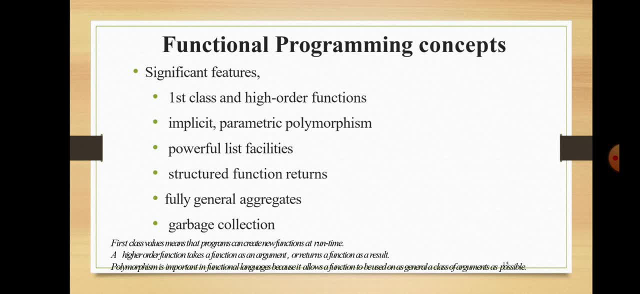 This is called first class function And higher order functions. Higher order function means we are giving a function as an input inside a subroutine, Or when we execute a subroutine, we get a function as an output. That is what we call higher order function. 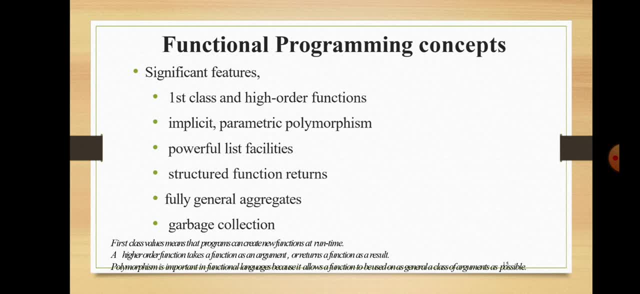 First class function means while at runtime we can create new functions. When we run we can create new functions. Similarly, in higher order function we can pass subroutines inside a subroutine. We can pass parameters inside a subroutine. We can't pass functions inside a subroutine. 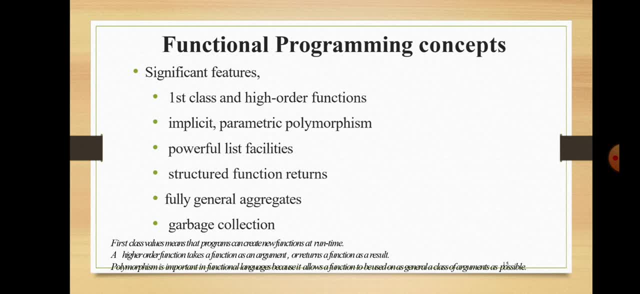 But there are cases. There are cases in which we can pass functions as parameters in the subroutine And also it can return functions as the result of the subroutine. It is made possible in functional language. It is possible in functional language. That is what we call higher order functions. 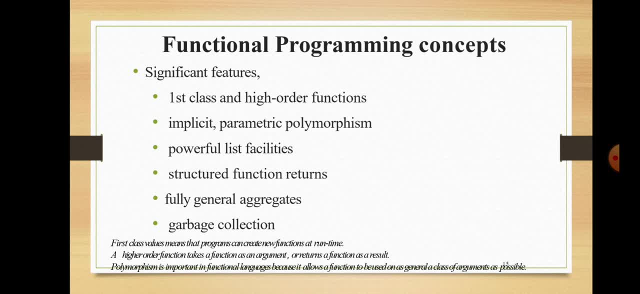 Higher order functions means what These are: functions which can take functions as input and sometimes it may produce functions as output. Such functions are termed as higher order functions, So it is a significant feature of functional programming language. Next is implicit and parametric polymorphism. 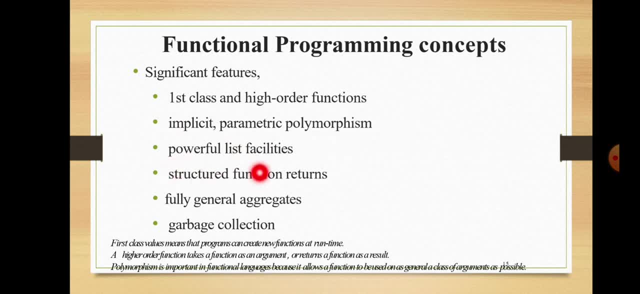 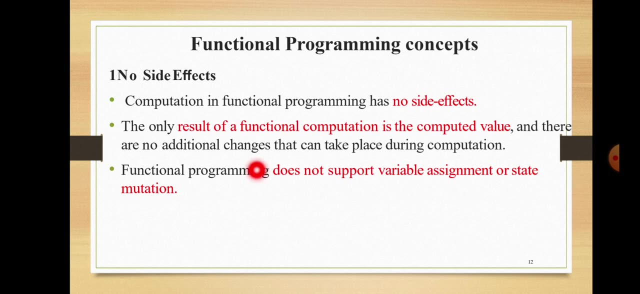 Then powerful list facilities, Then structured function returns, Then fully general aggregate, Then garbage collections. So these are the significant features of functional programming concepts. Next is no side effect. As we have already told, output means what? Output is always a mathematical function of the input. 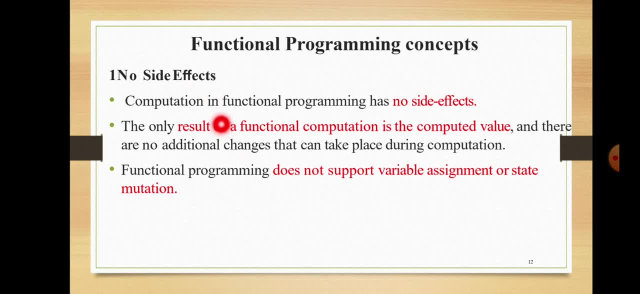 It means there is no internal state between input and output. Since there is no internal state between input and output, there does not exist any side effect. So computation in functional programming has no side effect. The only result of a functional computation is a computed value. 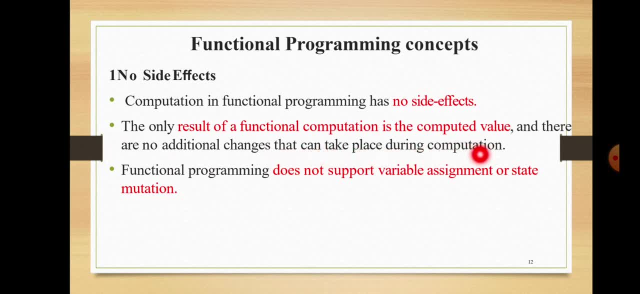 And there are no additional changes that can take place during computations. Functional programming do not support variable assignments or state mutations. When we give an input to a function, we get an output. What is there in between? There is no concept of temporary storage. 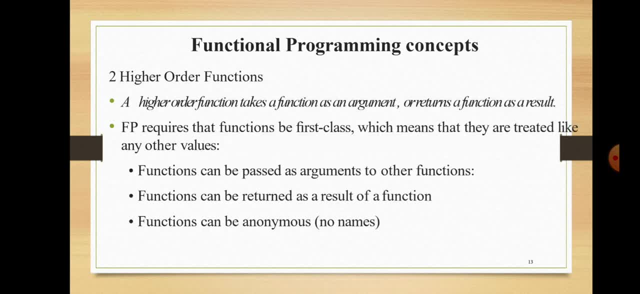 So there is no side effect. When we give an input to a function, when we perform a few computations, some other function is using that particular variable before completing the original one. So while a function is running, someone else is using a value. 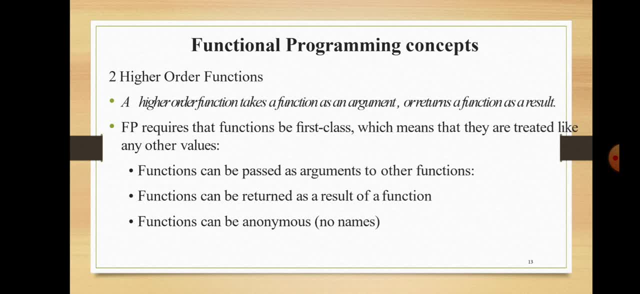 But the actual value is not available. There may be a possibility of a side effect, But in this case, in functional programming, the input is applied to a function. When that function is applied, we get the corresponding output. In between there is no intermediate state. 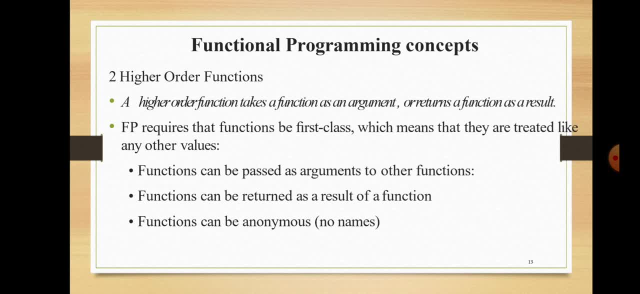 There is no intermediate state, So there is no side effect. Next is higher order function. Higher order function- I have already told it will take a function as an argument Here functions. Higher order function is a function which can take a function itself as an argument. 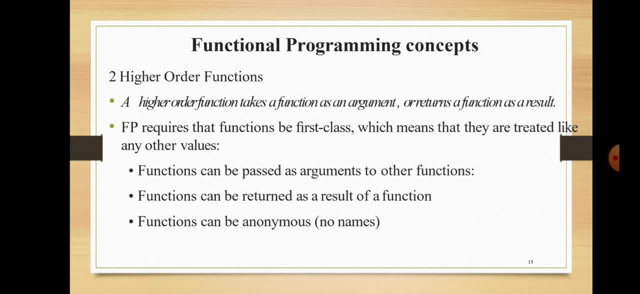 or return a function as a result. Okay, This concept is not possible without C. Without C, we can never pass functions as an argument. Now I have called a function called sum For that we can pass variables as parameters For that. 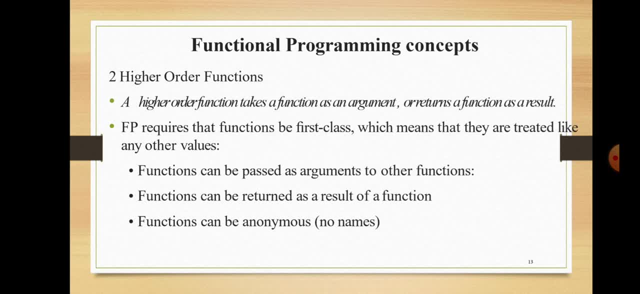 we cannot pass a function as a function. We cannot pass a function as a parameter or an argument. Okay, So this is also a major feature of functional programming concept. Okay, Next is functional programming requires that function be first class, which means that they are created like any other values. 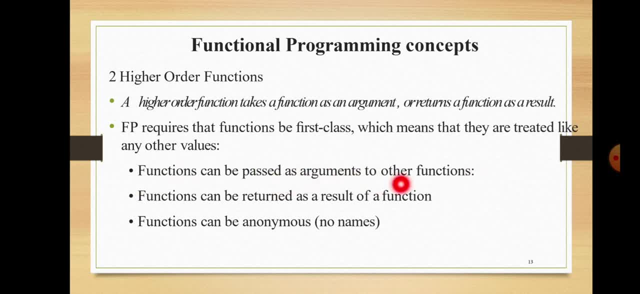 Okay. Function can be passed as an argument to other functions. Function can be returned. as a result of it, Function can be anonimous. Anonimous means that it can have no name. If there is a function, there should be a name for the function. 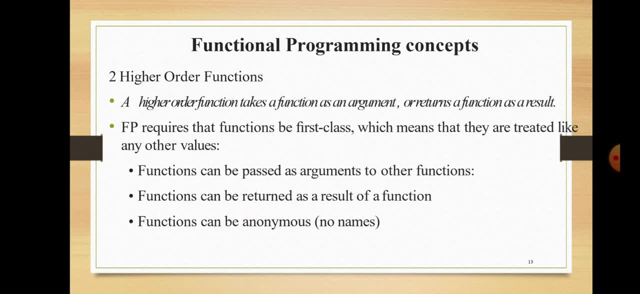 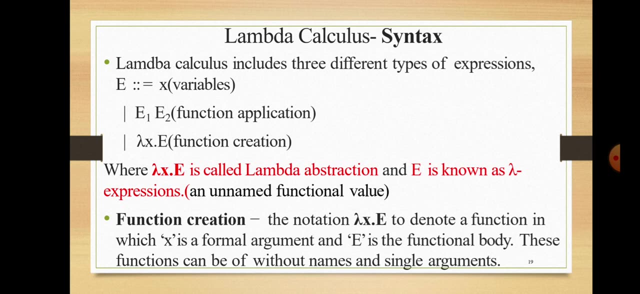 There should be a name for the function, But in the case of functional programming language, it is not such important that there should be a name. Nameless functions are also possible. Okay, So, as we already told, the word of computation behind. 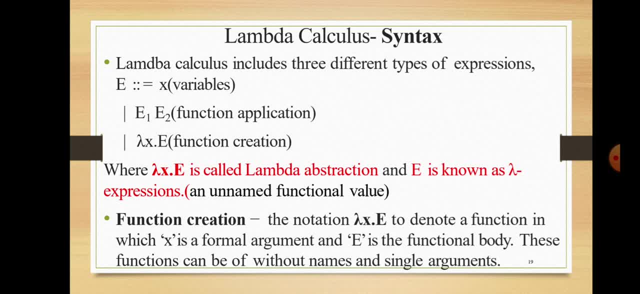 lambda. sorry, functional programming is lambda calculus. Okay, So now we are going to look into deeper about the syntax of lambda calculus. Lambda calculus can take any of the following three expressions. It can be any of the three different types. It can either be of this type or this type, or this one. 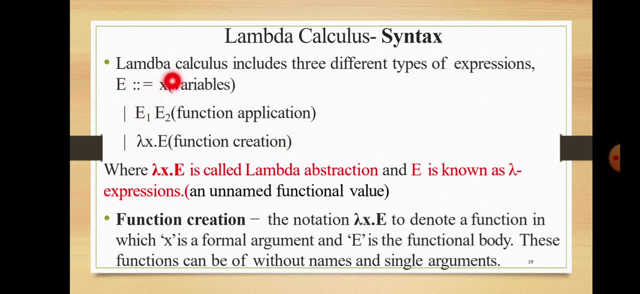 Okay, The first type is just expression equal to x, a variable Expression equal to x. Next Next type is expression is equal to e1 dot e2.. Not dot e1 e2.. Next is lambda x dot e. This capital E indicates always expression. 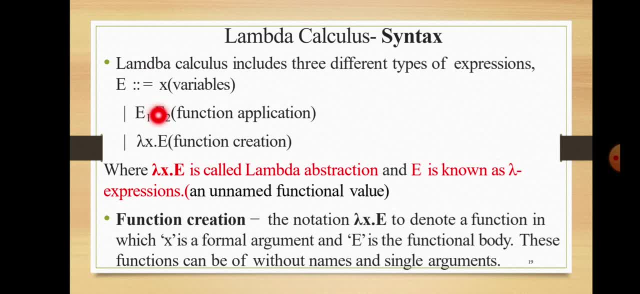 Then x should be variable, or parameters or arguments. Okay, So the idea for this equation is to get the function of all these three numbers. So what do we do? We goes like this: If e is the lined up point and D is the starting point, 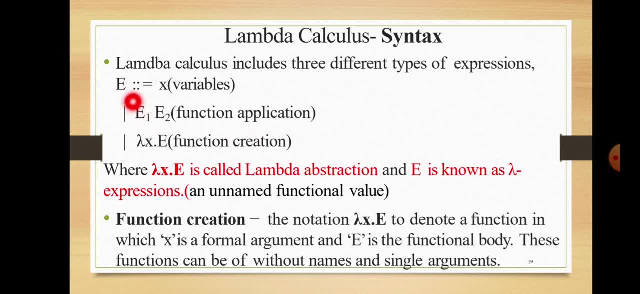 pole that extends from that point Now is called a stagnant line. It has expandingpldır And then the situation is XX. So lambda x dot, e is called lambda abstraction. This is what we call lambda abstraction, And e is known as lambda expression. 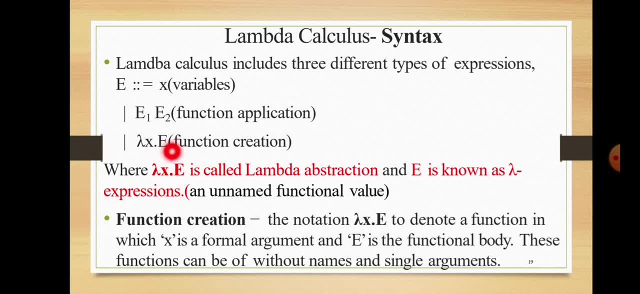 This is what we call lambda expression. Next is function creation. We will look at this in depth. This is the notation: lambda x, dot e to denote a function. This is denoted by a function function. lambda x, dot e A function: This function is denoted. 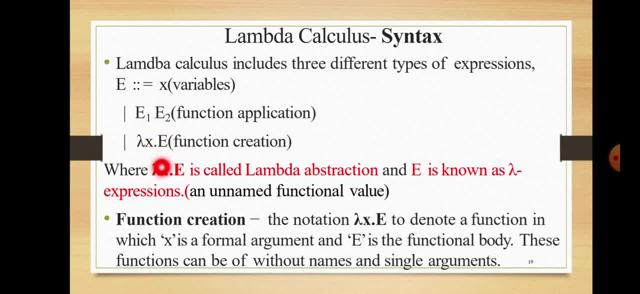 Inside this x is called function. What comes to the function? c, Parameters come to the function. Parameters come to the function. Then the steps that are done by the function come. x is called parameters. formal arguments: E means it is a function body. 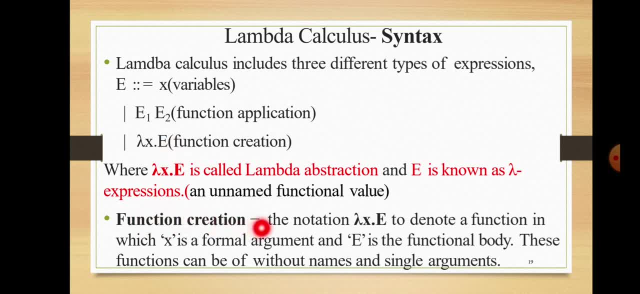 These functions can be of without names and single arguments. We don't need a name for functions with lambda expressions. We can write lambda expressions with only single arguments. So lambda calculus is the basic idea behind functional programming languages and it can take any of the three types. It 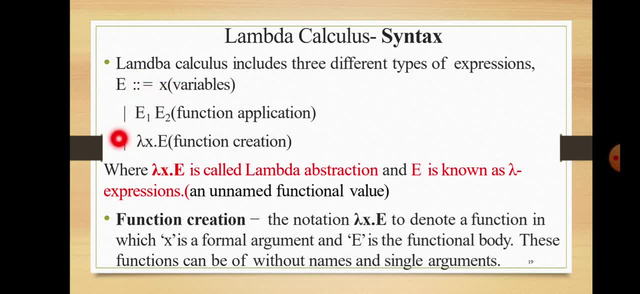 can either appear as expression is equal to a single variable, then expression is equal to expression 1, expression 2 is no longer allowed to be discussed here. ISS is lambda. xE, fraud, Y is the第번째apa dancing Law that we are discussing now. that is function. 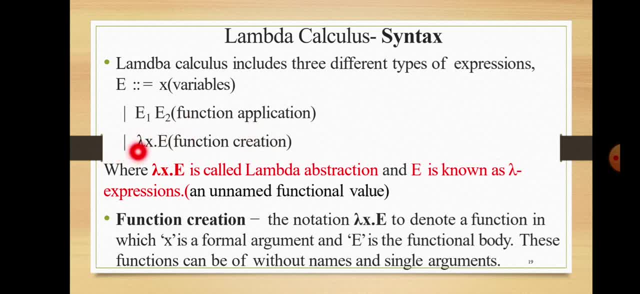 creation 08: DAVID그ی. in the indicator and it's a lambda calculus means it's a function lay nameless function, animal lambda calculus number. I'm gonna get off the lambda another indicating it's a function. it's another, another formal parameter, then E and over another it is the board. it is a function body, okay. 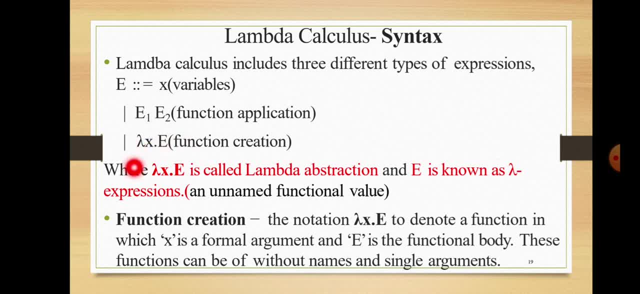 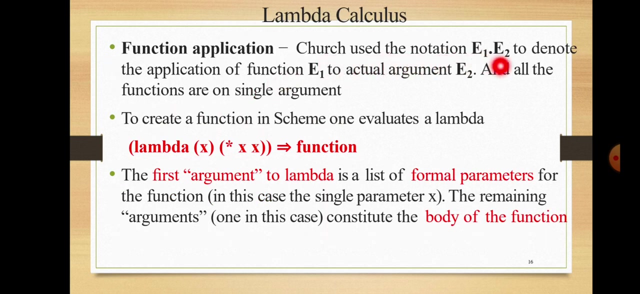 about: lambda, indicating it is a nameless function. X, indicated to another it is a arguments or formal parameters of that function. then E, indicated saying that it is the body of the function. okay, next is applicant function application. this one function application search, uses the notation even dot e2 to denote 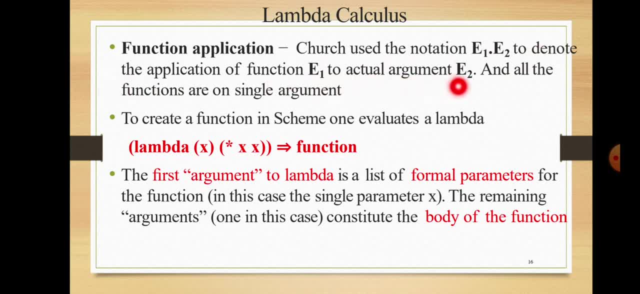 the application of a function even to actual argument e2 and all the functions are on simple arguments to create a function scheme. one evaluate a lambda expression in a curio function creating and function protects the other name in your curriculum about nameless function number and don't indicate in lambda in the one. 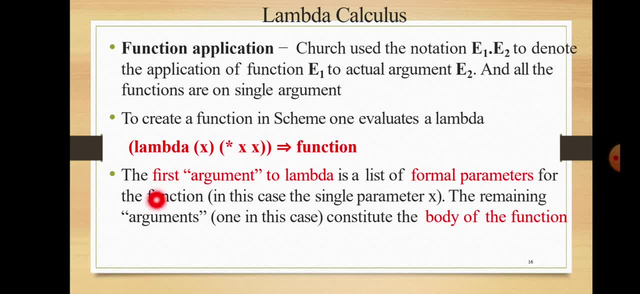 indicated just lamp and they could open all the protects the other in a moon curriculum. so lambda then. X isn't the indicating of the. it indicates either: this is a formal parameter. next, indicate: either this is the expression yeah in the day it on a formal parameter, in it on a body of the. 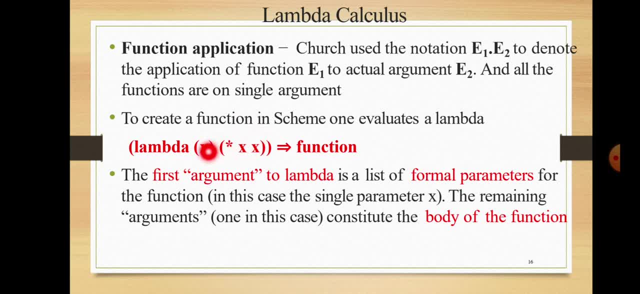 function that if it's a and I'm gonna come down a number, edit in the parameter and the square and number to come. now that is star XX, means it's a prefix notation. I like the otherwise termed as Cambridge Polish notation nameless scheme. I like Lisbon, the one a program in language lay. normally use the. 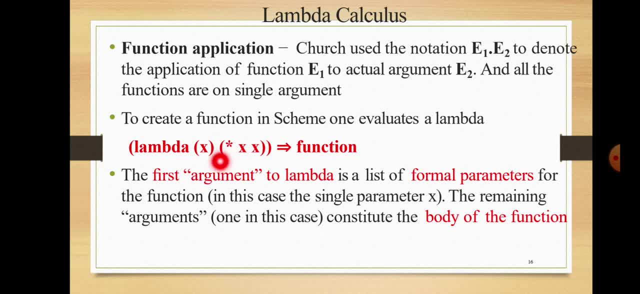 chain a notation or another prefix notation and our support in a zone on a English okay scheme support Cambridge Polish notation which is a version of prefix notation okay. so this is a lambda expression or function in scheme and again that we did really in the square of a number car. I made it a lot of fun starting any. 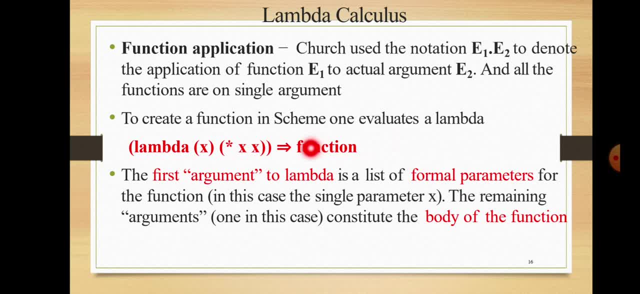 ridiculous. now our function. it protects the name on the God of vanilla. just a lambda and matri. you know what a number in the square, car, no angle, which, if the arguments are passing, I'm wouldn't have been. the square, a gondola, so we should. 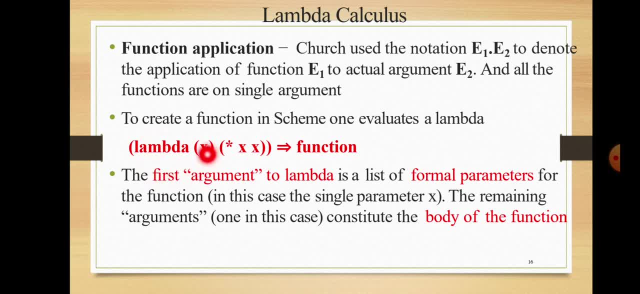 have to pass only a simple argument. so that argument is X, then in a chain, the step and on and on, thrive X in a tendu portion multiply, that is actually X, a star X, but screen support prefix notation, so it is written as star X, X. star X is none of individual. 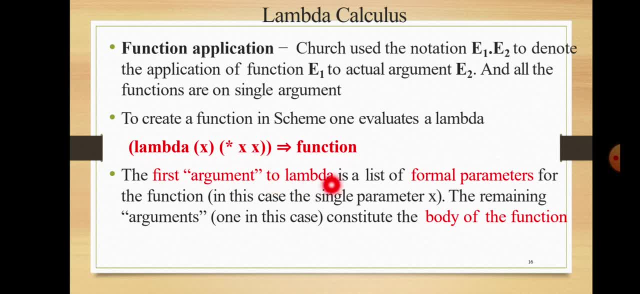 okay, so the first argument to lambda lambda lot love. first argument in the. what I know, it is the list of formal parameter. palzenbel¡¦ artist argument. this one in all ran of the list of formal parameters: ek8, constitutional formal parameter. matre- ok for the fun, in this case, the single parameter X. after that. 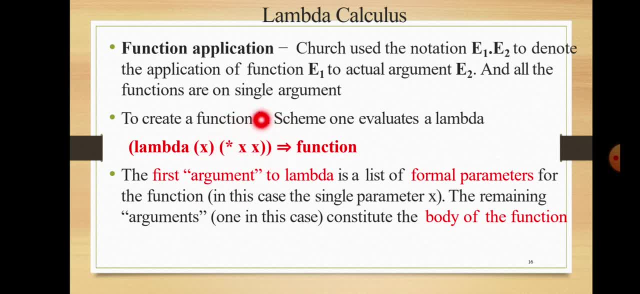 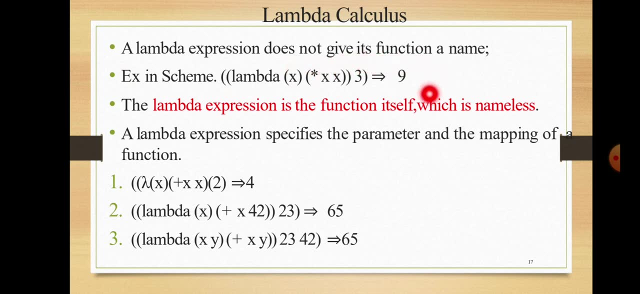 remaining in the variety, the expression or body in the variety: ok, the remaining argument: constancy: body, ok. body of the function a lambda expression does not gives its functionally lambda expression would kill him a function, a door. gila name go to gila, okay. in the epitome number expression: link, a link load. 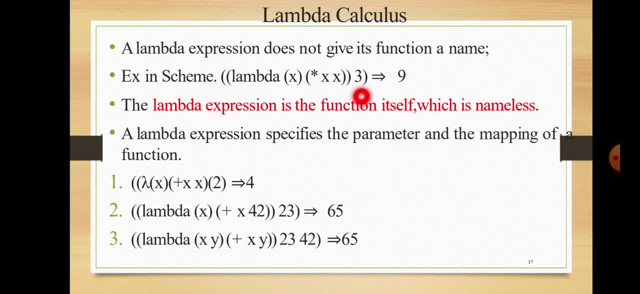 function scheme: leprosy: normal: a function or another parent. this is not the diagram. okay, within the parent. this is okay. you would adjust to no, no key. a lambda expression is the function itself, which is nameless, but I just don't know car. so the connect. you would a double bracket and I'm gonna look under just 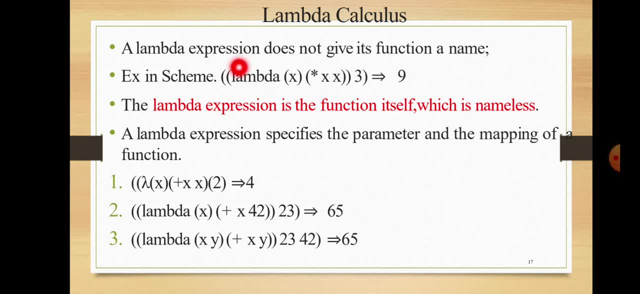 in an argument in there, you know. next for you, function on it, I'm gonna shoot you. it should be given in bracket. so now the way outer bracket in Okinawa lambda could talk to me in your bracket, bracket, lambda, over a square and in the conda. so 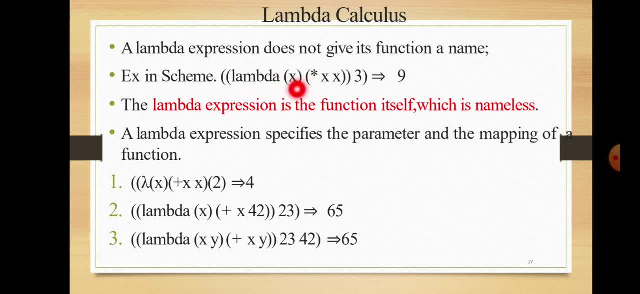 a single parameter, Adam, or the bracket, then parameters of. the next is the body of the function. so again, bracket, star, X, X, that bracket close, you know. then, lambda, close the new. now I am passing a value, or binding a value to the space, a eingo nerd value, parity. it should also. 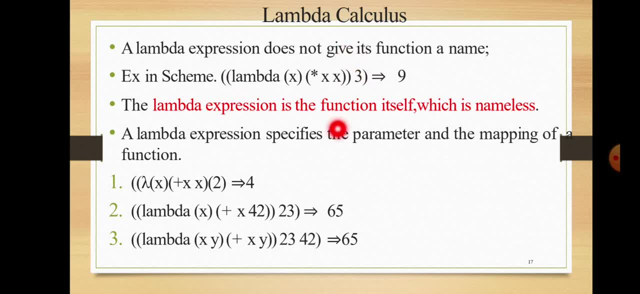 be given in a parent. this is, add a number of worksheet, kaara. so while executing this state or this function, X will take the value 3 and produce 3 star 3, which is man. ok, I will Starting in your banana lambda. either have a bracket at this bracket open to the lambda in equal to square of. 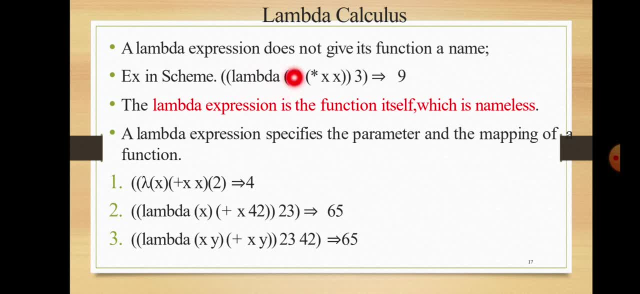 Then lambda square of a number means 9.. currently the sole is single parameter. parameters to number in the list of parameters I'm gonna bracket equal to: okay, then the body of the expression. again other normal bracket equal to. so bracket star xx are the closer to lambda. 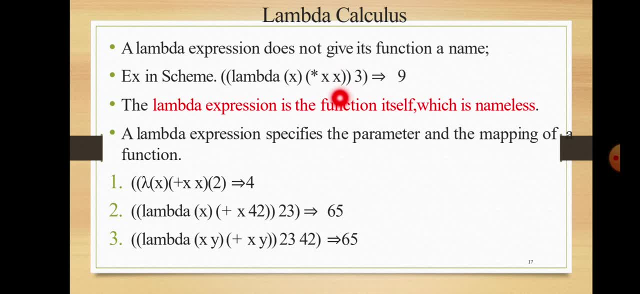 and close either. now I am passing the value along with. this is no good the node upon the name value passing. so it should also be given in brackets. so bracket 3, bracket okay, so 3 does square, nor another. 9, the lambda expression itself specifies the parameter and mapping of a function. if it a lambda in. 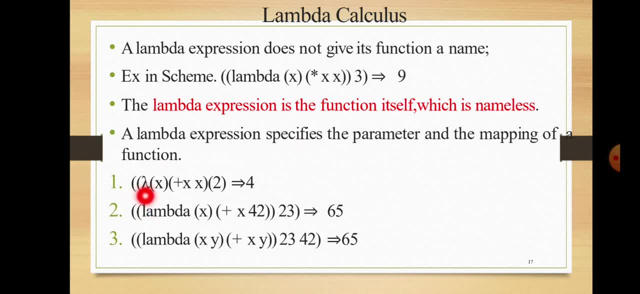 over another lambda in the code current, in just a lambda to symbol go table. okay, lambda, every single parameter. you know then the steps I want to do is I have to add, add, yeah, so prefix notation and plus xx, okay, then your value, bro, could go to okay, so it will produce a result for next is: